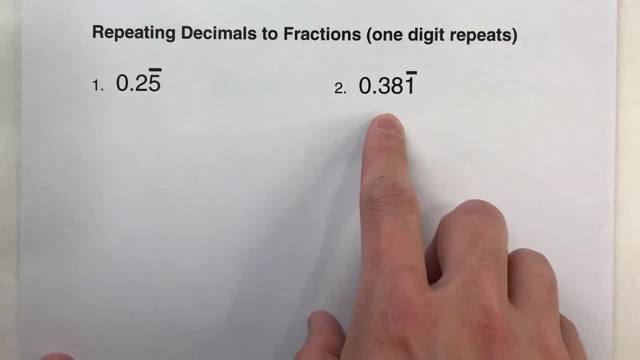 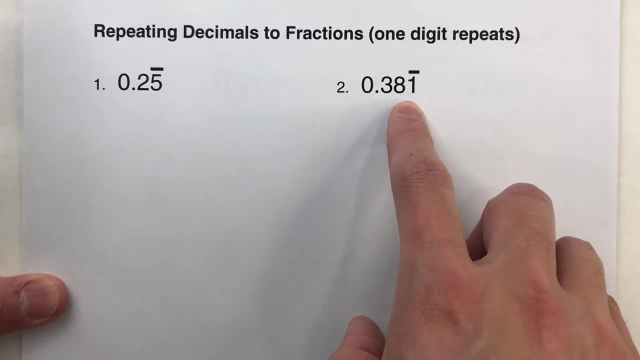 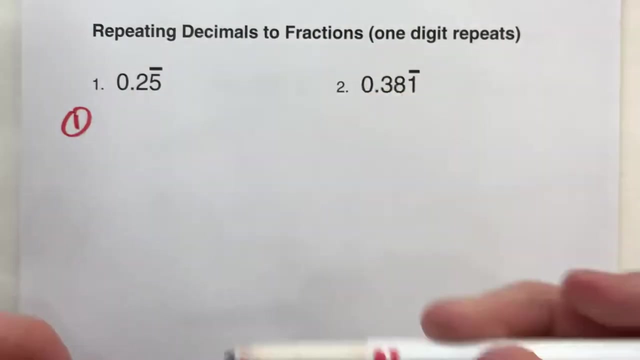 So today we are changing repeating decimals into fractions, or specifically repeating decimals, where just one digit in the number repeats. all right, and i'm going to break it down to you in four steps. all right, so step one: what we're going to do is write an equation using x as the number we're. 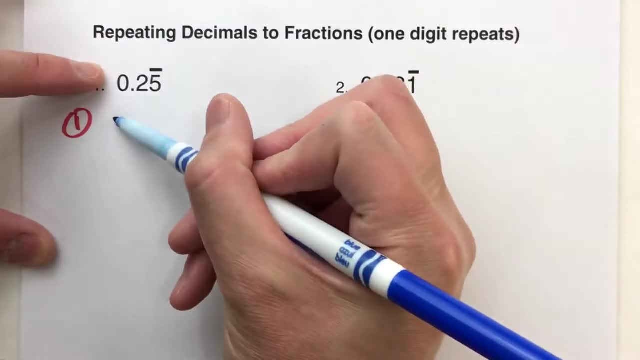 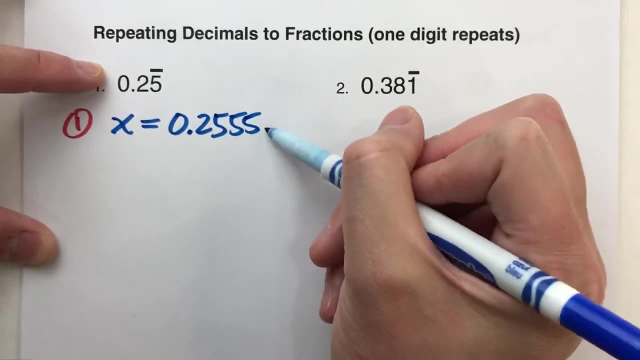 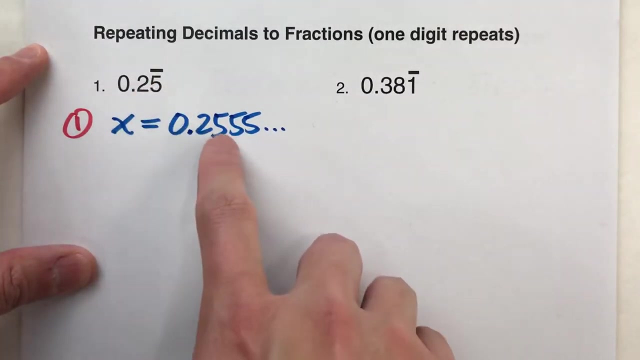 trying to find. so, in this case, 0.25, repeating- i'm going to write x equals 0.2 and i'm going to write it out kind of the long way: five, five, five, five, five, five, five, dot, dot, dot dot. all right, because that's what this represents. it's 0.2 with a bunch of fives after it. all right, step two: we're going. 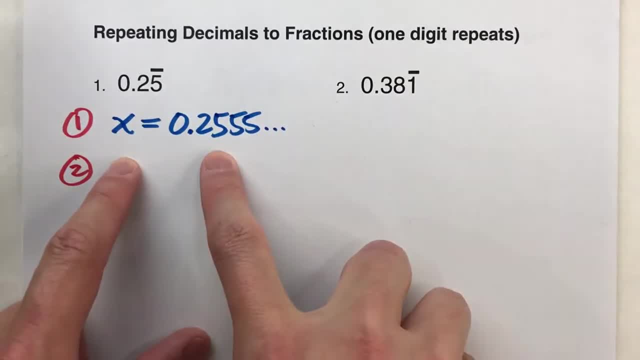 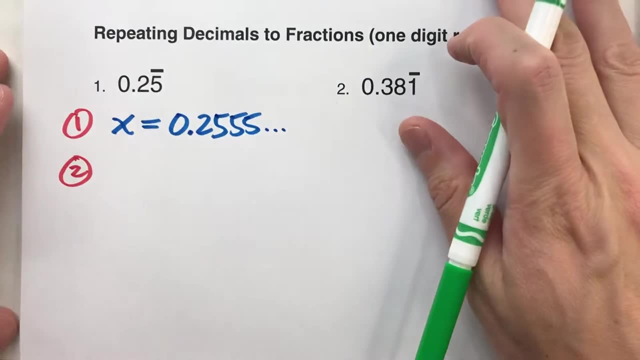 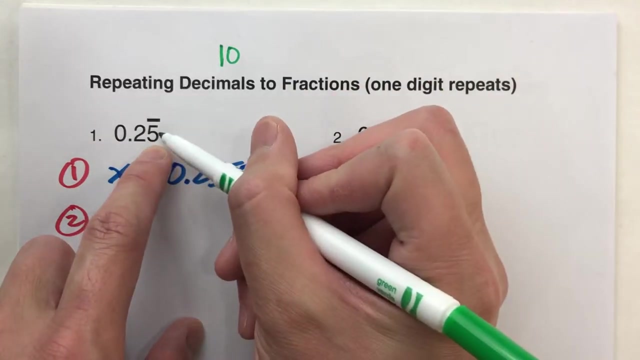 to take this first equation and we're going to make another equation out of it, my, by multiplying both sides by a number. well, what number specifically? we are going to go 10 to the power of however many digits are repeating. in this case, just one digit's repeating, so that factor is going to be 10 to the first power. 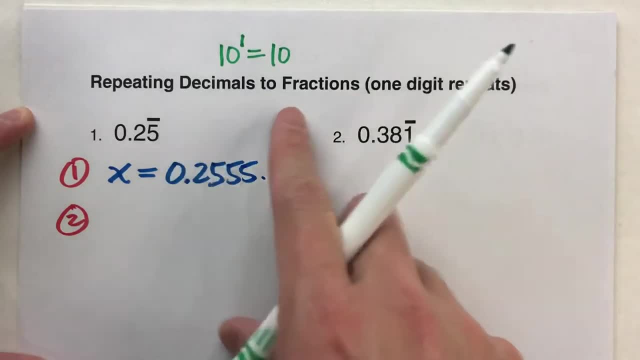 which is 10.. all right, now, in a different video, i'll show you examples where there's two digits repeating, and three digits repeating in that case would be 10 to the second power or 10 to the third power. luckily for today, only one digit's repeating. 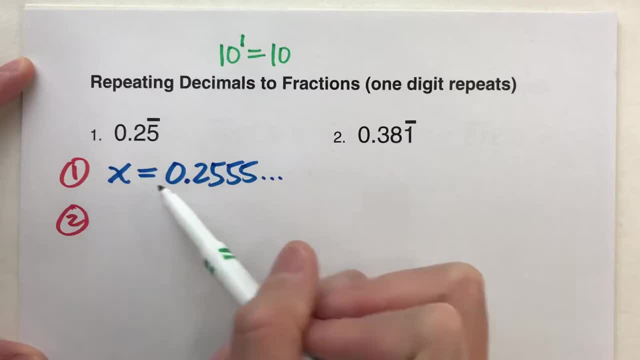 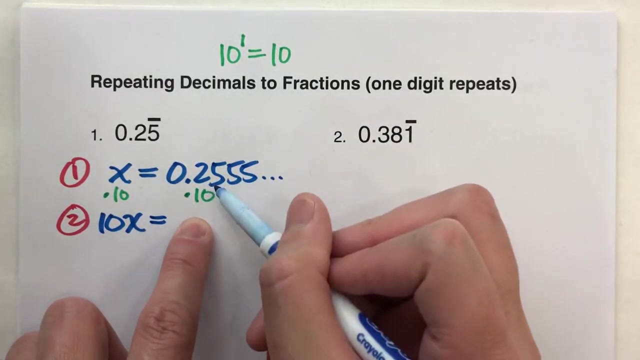 so it's going to be 10 to the first power. so i'm going to multiply both sides of this equation by 10.. all right now, when i do that, 10 times x gets me 10x equals. if i multiply this side by 10, i basically just move the decimal place over, so that decimal 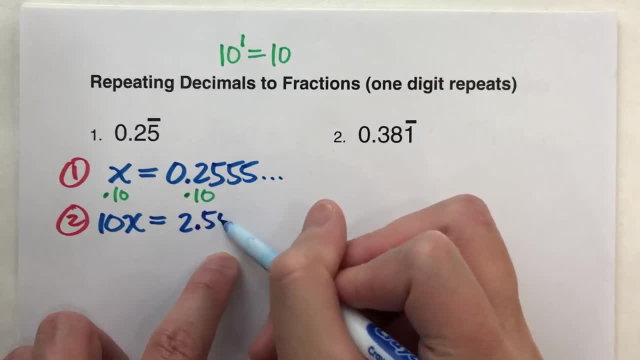 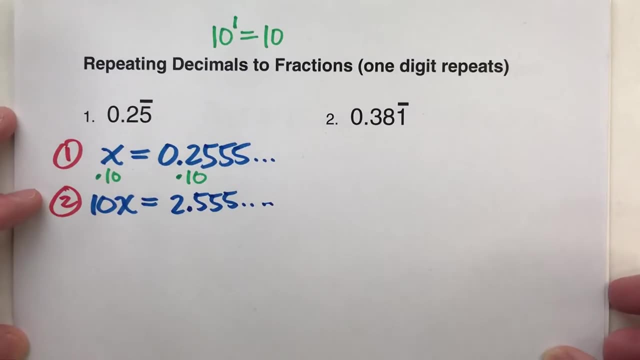 is going to move over. this is going to become 2.55555, repeating forever. all right, so i just ended up making a second equation that doesn't look that different than the first equation, all right, so the first two steps are done. step three now. what we're going to do is take this new equation and 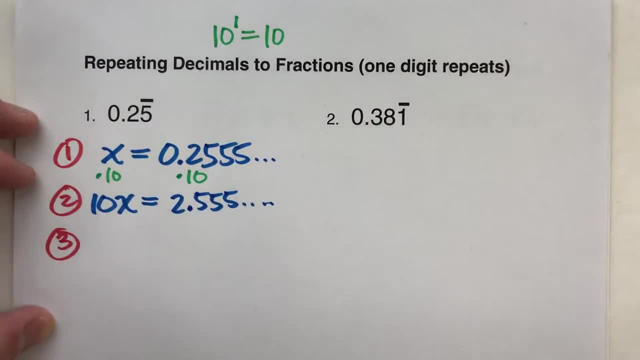 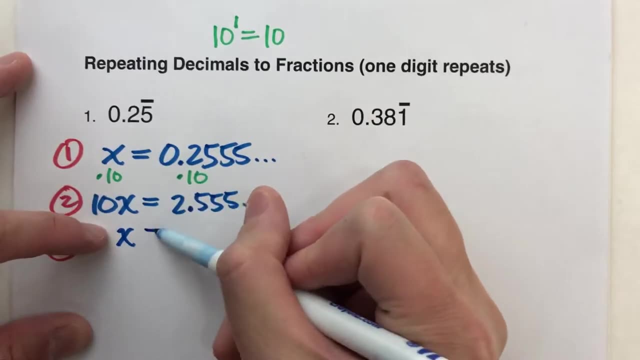 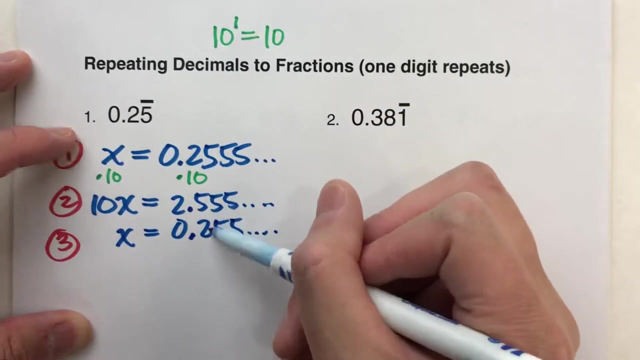 subtract the original equation from it. all right, so what i mean by that is: i'm going to take that original equation, write it underneath here: x equals zero point two, five, five, five, five, repeating. i don't need that last five because i want them to line up with the other one so that the decimal 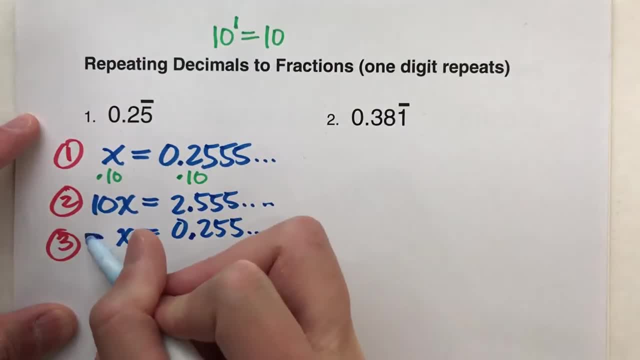 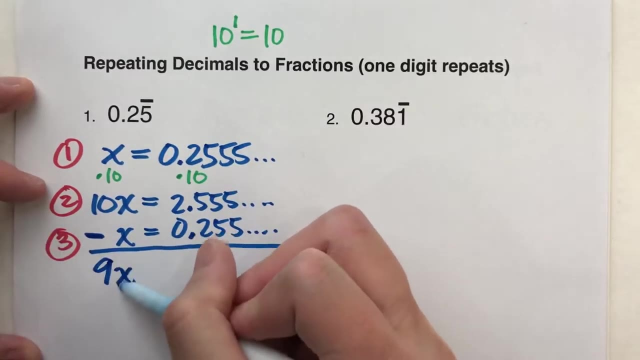 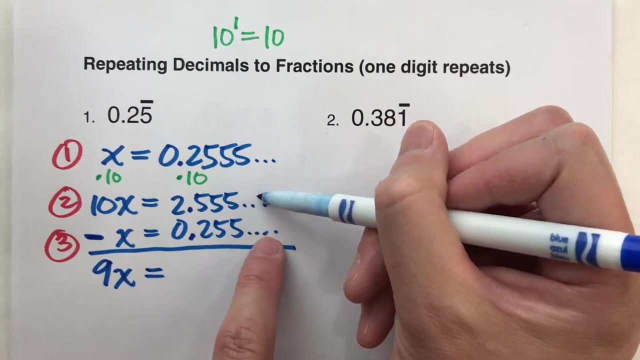 place lines up over here, because we're going to subtract these two equations. all right. now, when i do that, what ends up happening? well, 10 x's minus 1x gives me 9 x's. on the other side, when i subtract these, notice all the digits are going to be repeating. 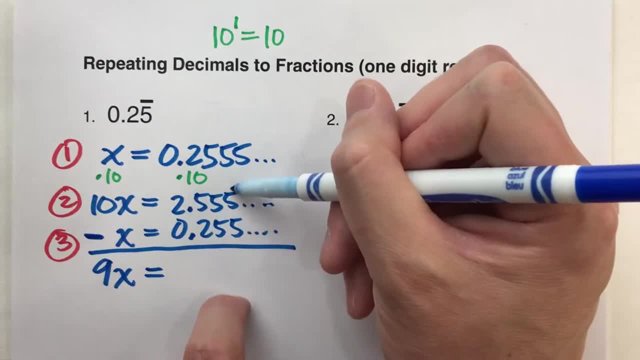 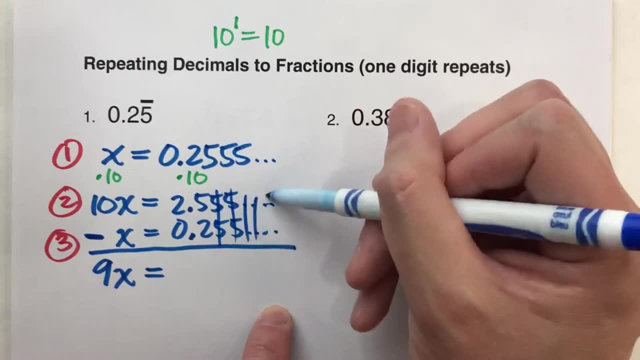 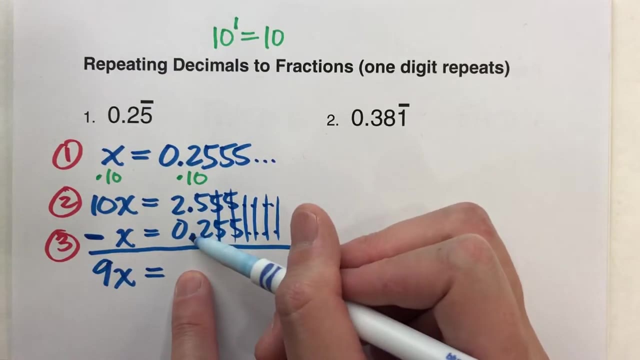 fives. and we know: five take away five is zero, and five take away five is zero and all these other fives are subtracting fives from it. so all of these are going to be zeros too. so all of these are zeros. so i don't even have to, i don't even need to write them down, because after the decimal, 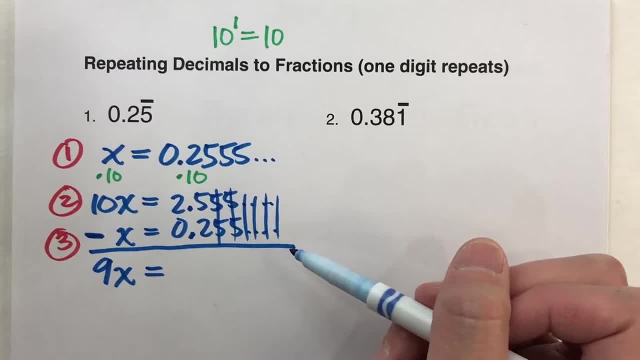 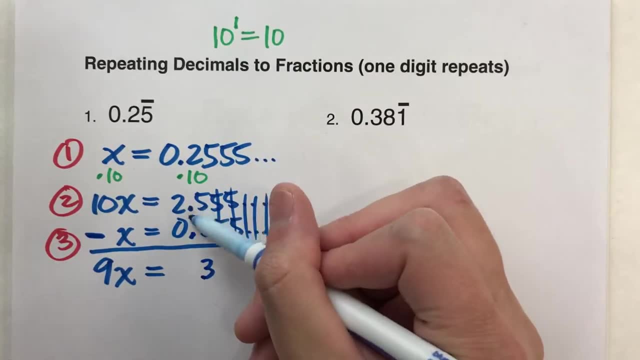 point. anything that's a zero is just not even going to be written. so really, all these five subtract off, all i'm left with is five minus two, which is three. drop down the decimal two minus two zero is two. when i subtract these repeating decimals from each other, i end up with 2.3. 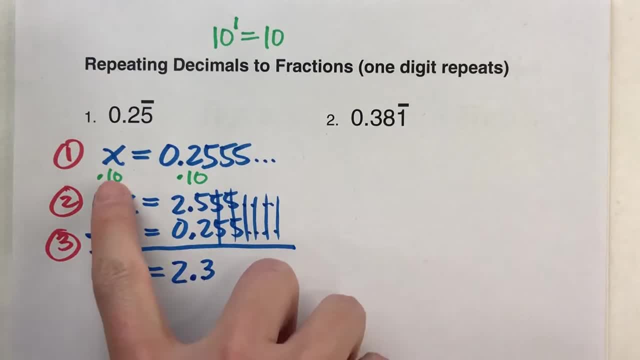 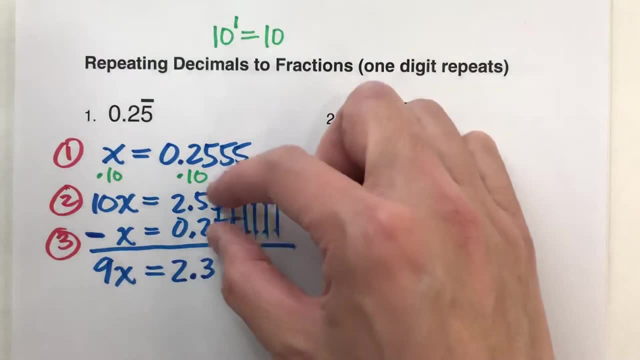 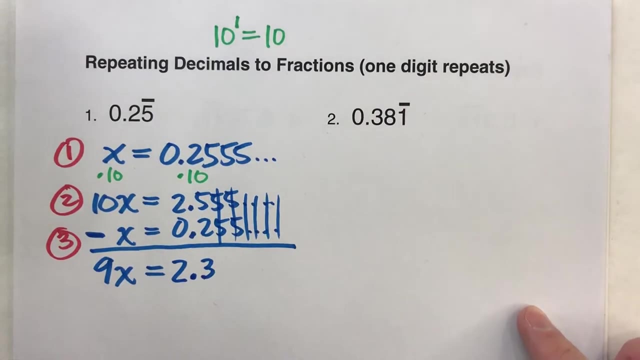 all right, and that will always happen, because when we multiply that first equation by 10, all we did was shift the digits over. but remember, all the digits that follow here are all fives, so they're always gonna be subtracting each other off and there'll be nothing left. all right, so last step. 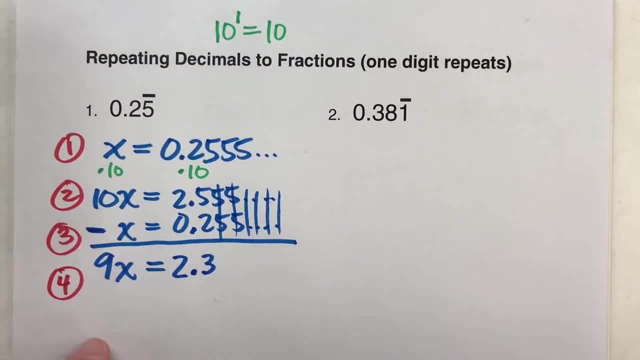 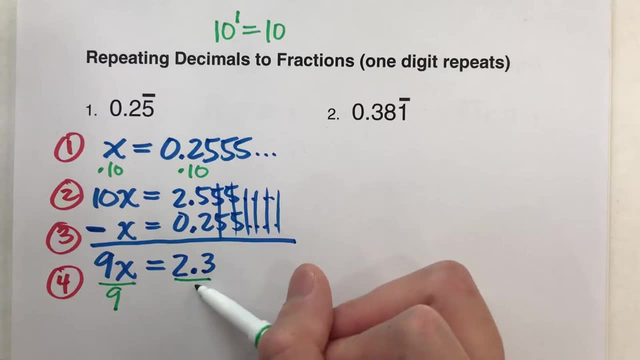 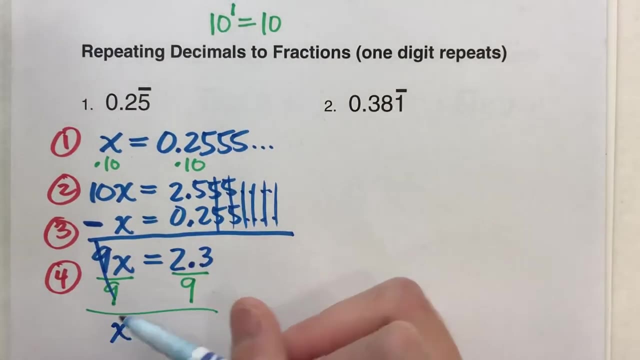 four, we solve for x and then simplify our fraction. i want to get x by itself. it says x times nine, so i'm gonna divide by nine. what i do to one side, i have to do to the other. all right, let's see what happens. the nines undo each other. x drops down, equals drops down. and remember, i want to keep. 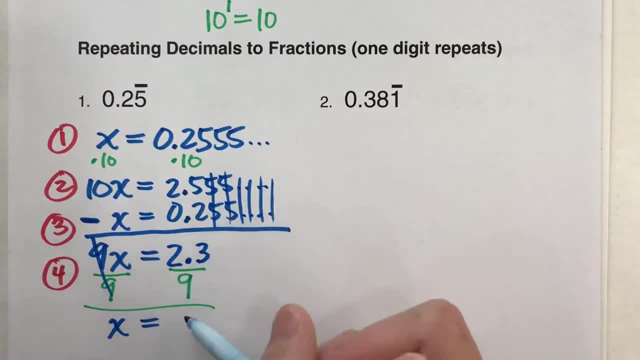 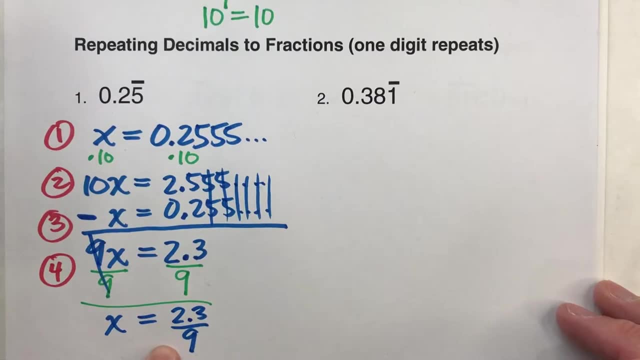 my answer as a fraction. so i'm going to keep 2.3 divided by 9 as 2.3 over 9.. all right, now one last thing. we have to sim. we have to simplify this and we're not allowed to have decimals on a fraction. so to multiply the top and bottom by a number to make this into whole numbers. 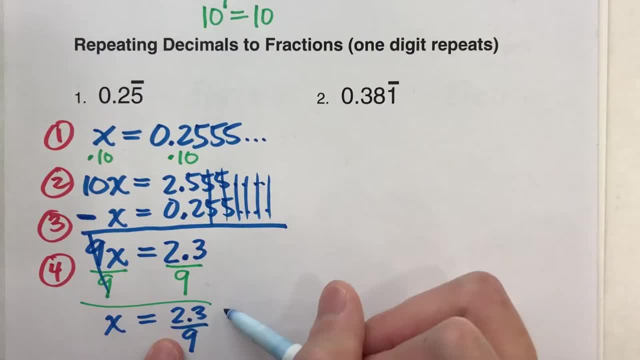 we have to be a little strategic. all right, i know if i multiply any decimal by 10, it'll move the decimal over. so i'm going to multiply the top and bottom of this fraction by 10.. and look what i get: 2.3 times 10 is 23.. 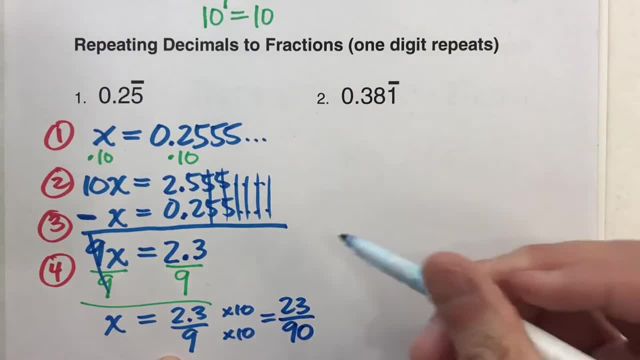 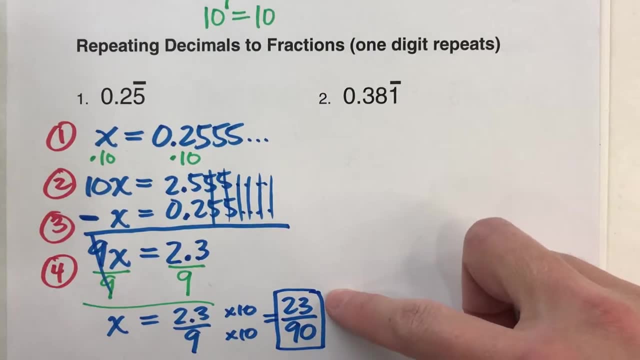 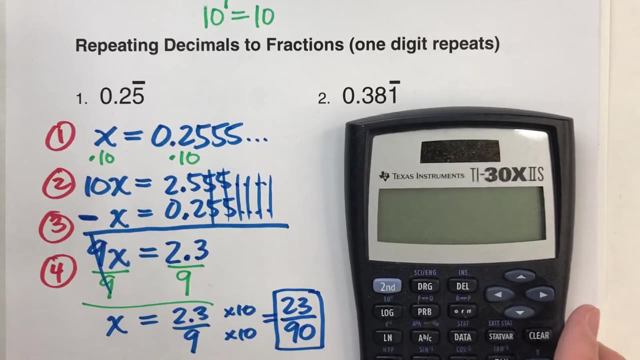 9 times 10 is 90. and there's my answer: 23 90ths. all right, and you should probably check to make sure you can. you can't reduce this in this case. i can't. i know 23 is prime, but you can always check. 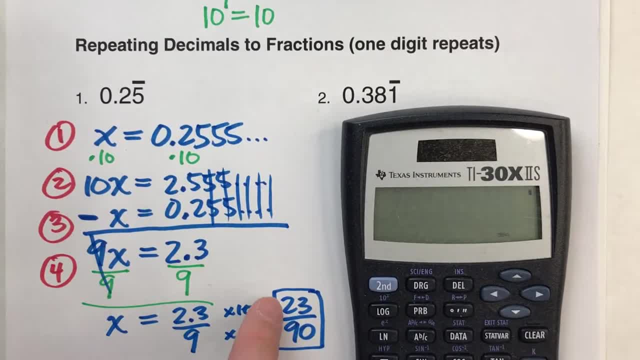 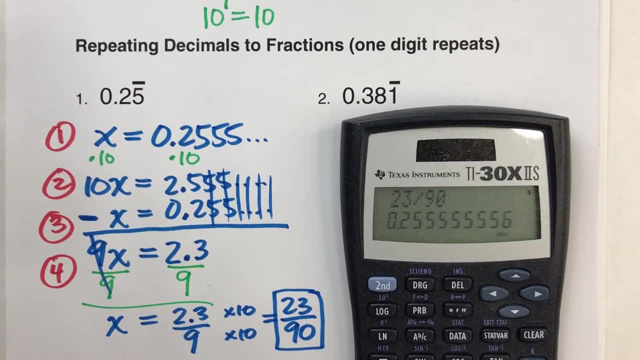 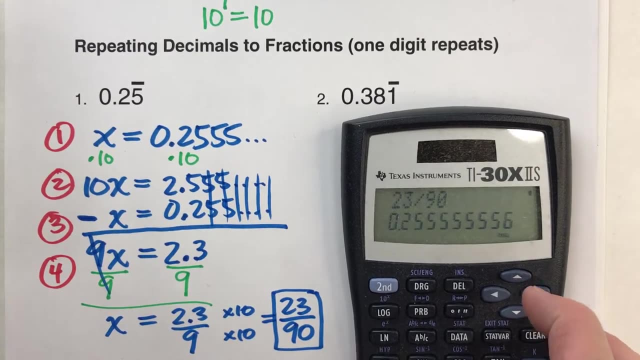 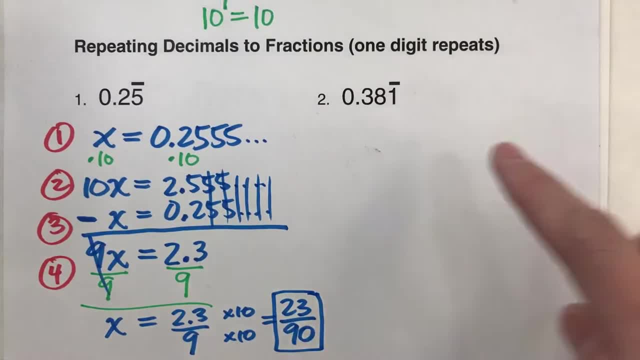 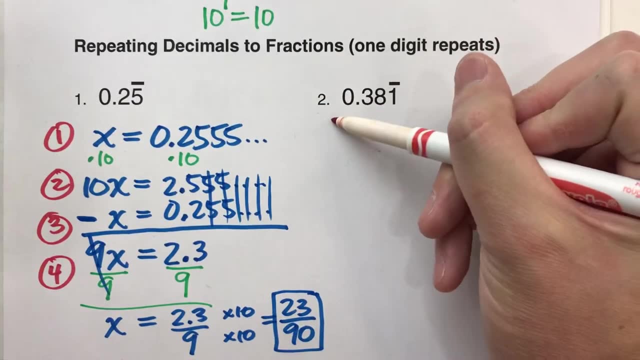 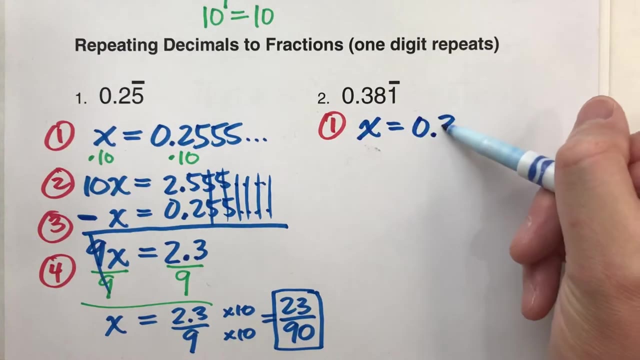 more time. this one's a little bit harder, okay, so again we've got 0.381 repeating and there's only one digit repeating. all right, so step one: write an equation: x equals that number. zero point three, eight, one repeating one, one, one, dot, dot, dot dot. step two: 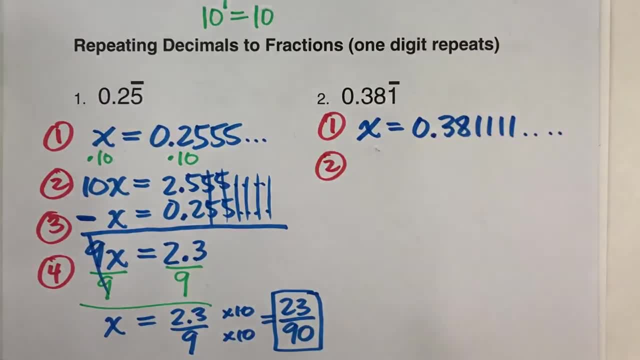 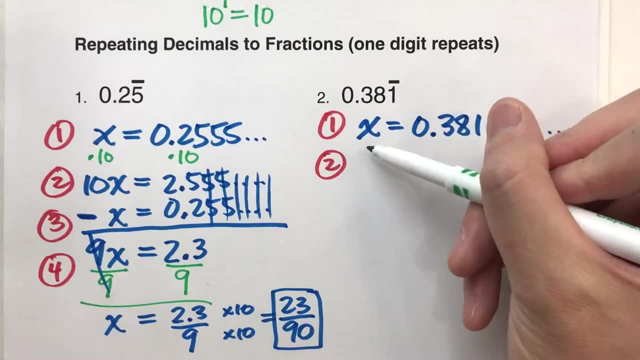 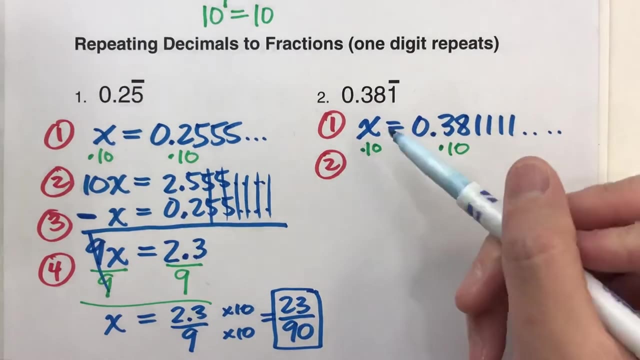 we're going to multiply both sides of the equation by 10, because there's one digit repeating and 10 to the first power is 10.. so we're going to multiply both this- the left side and the right side- by 10.. and when i do that, 10 times x gets me 10x on the other side, if i multiply this by 10, i 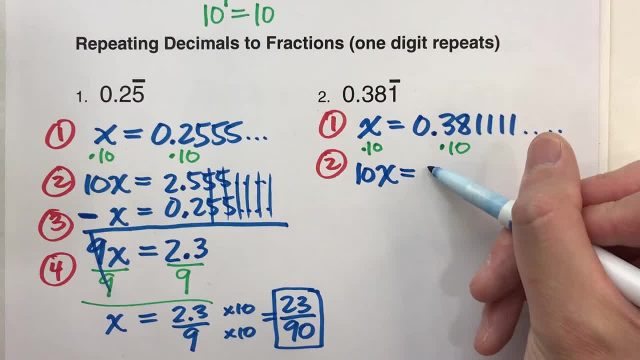 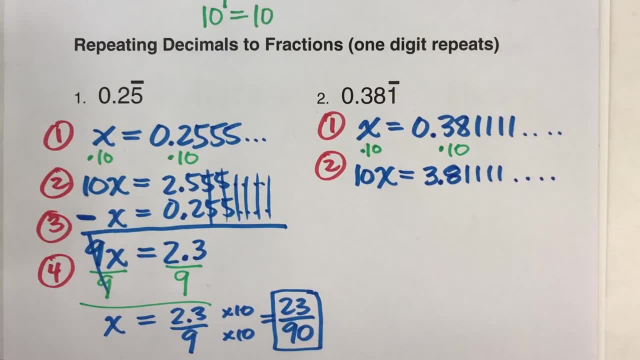 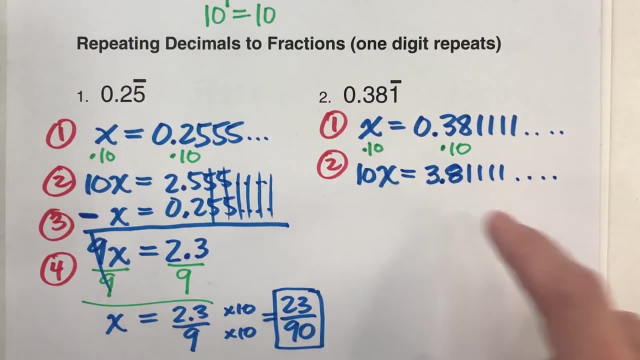 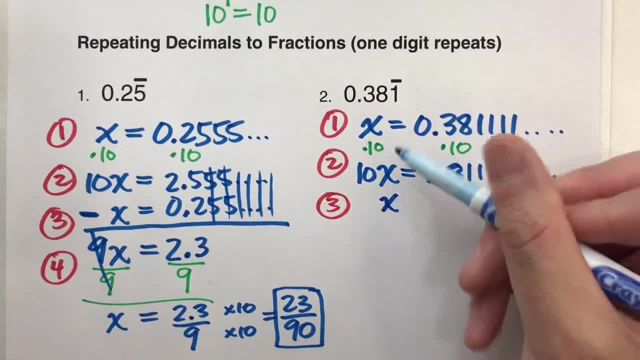 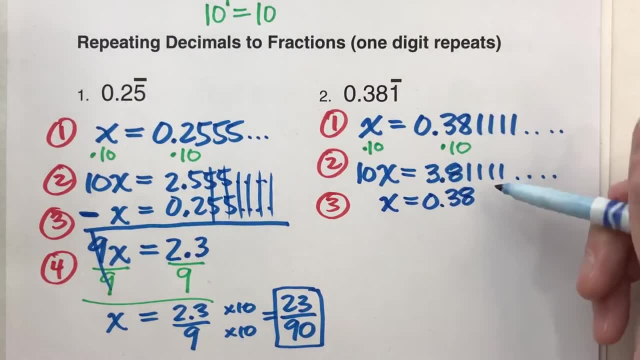 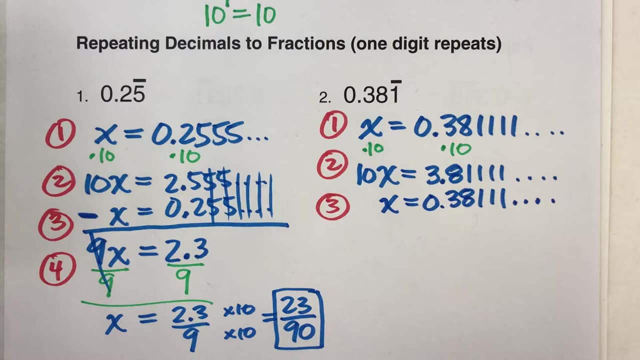 take that first original equation that x equals zero point three eight, and notice i do line up the digits because i know i'm going to subtract later, so it makes it easier on myself if i line up those digits. okay, but i'm going to go ahead and subtract these now. all right, so when i 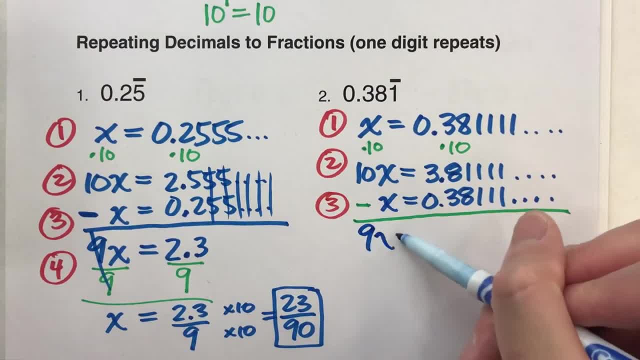 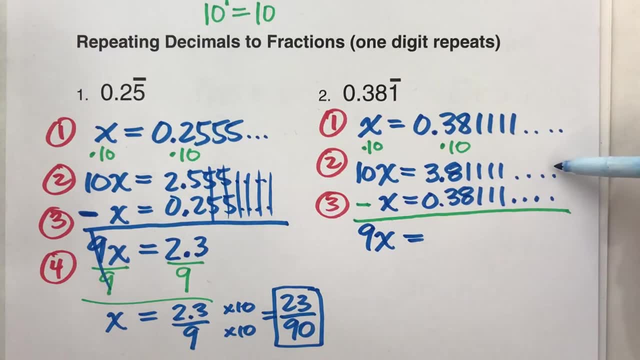 do that. 10x is minus 1x is 9x. on the other side, now when i subtract, i know all these ones. i've got ones on the top and ones on the bottom, so they're just going to subtract to 0 because 1. 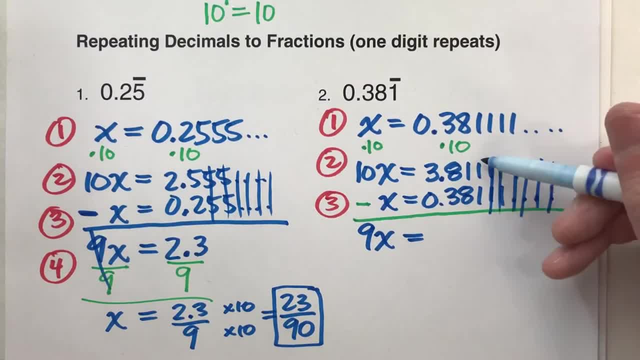 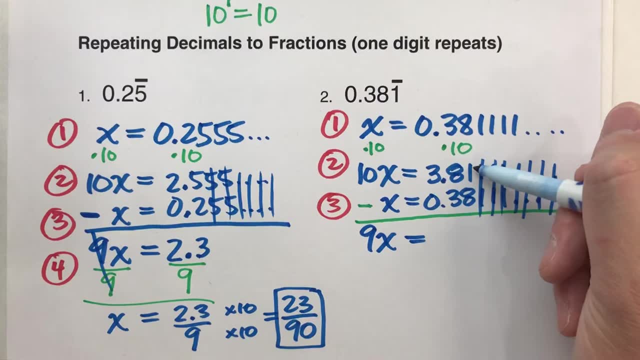 minus 1 is 0. 1 minus 1 is 0. all the way down here until i get to this point, all right. and then i have to really subtract, all right. and you have to remember you can't do one takeaway eight, so you gotta borrow from the eight, make it a seven and put, oh uh, one there. so we've got eleven, eight. 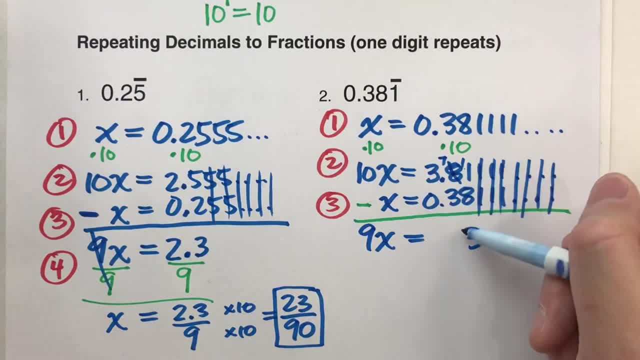 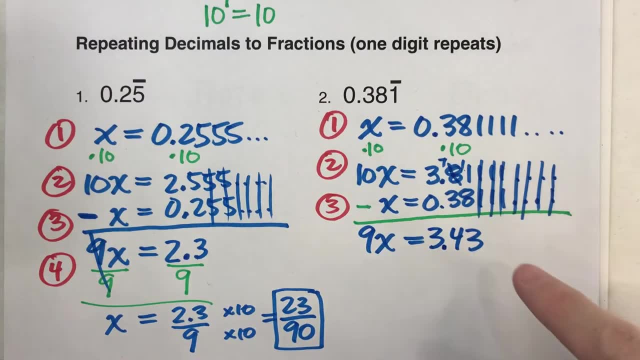 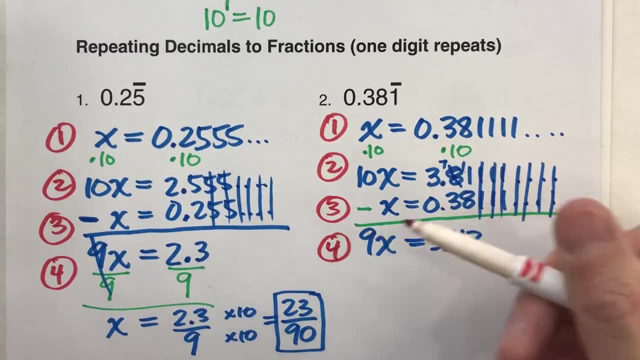 eleven minus eight is three. seven minus three is four. drop down my decimal. and three minus zero is three. okay, and if you can't remember how to subtract like that, you can always use your calculator to do that. but we're almost done, because step four, solve for x and simplify your. 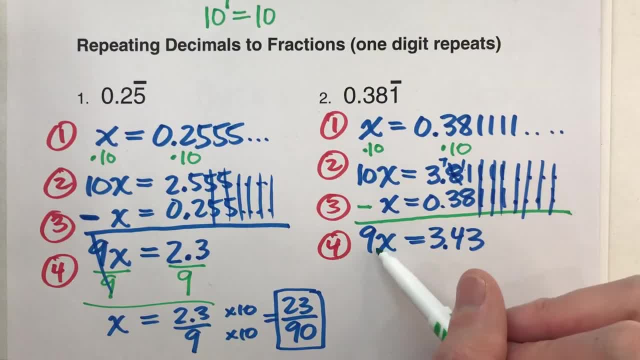 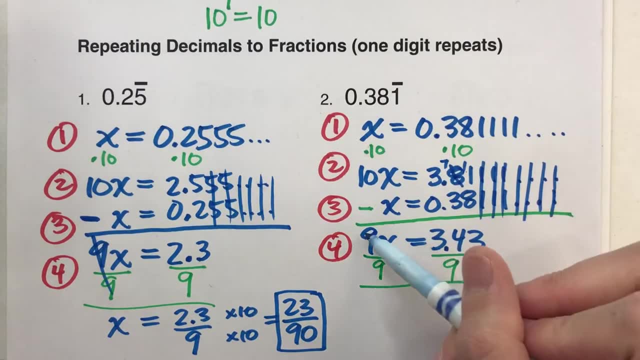 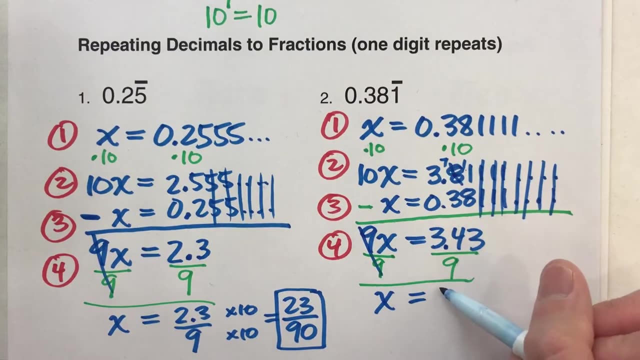 answer by dividing both sides by a fraction. to get x, i need to divide both sides by nine. all right, and once i've done that, the nines undo each other. x drops down, equals drops down, and i want the answer as a fraction, so i'm going to leave it like this: 3.43 divided by 9 is the same thing as 3.43. 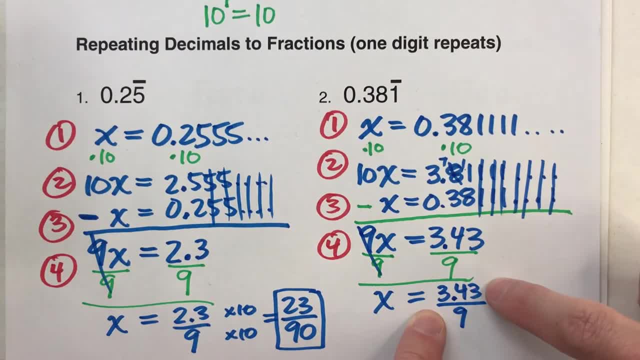 over 9.. all right, but like we said before, you're not allowed to have a decimal inside of a fraction. i'm going to multiply it by something to move that decimal over and make it a whole number. now, in this case, i need to move the decimal over two spots. before i only had to move it over one to. 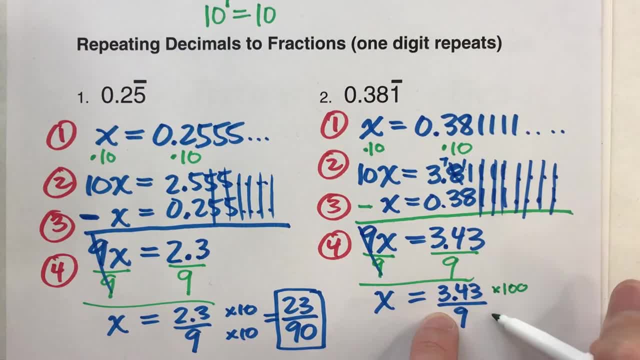 move it over two spots. i'm going to multiply the top and bottom by 100, because, remember, when you multiply by 100 it moves the decimal over two places. so 3.43 times 100 gets me 343.. 9 times 100 gets me 900. 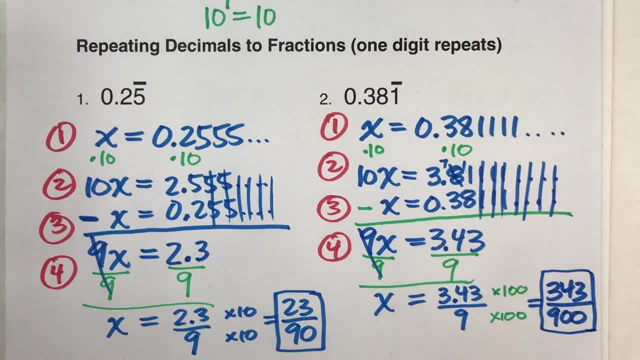 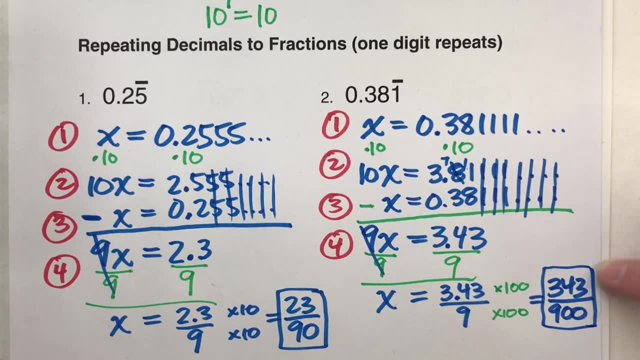 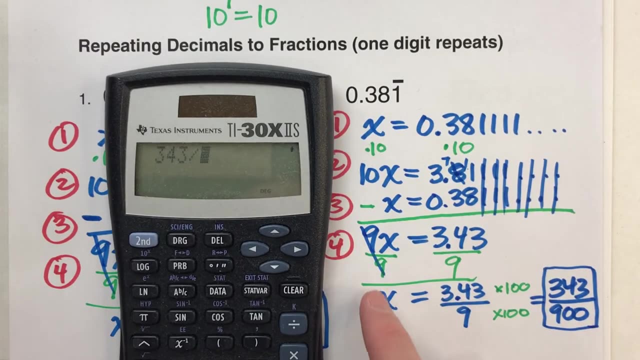 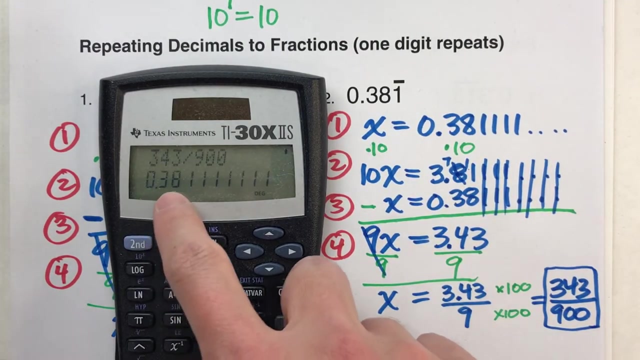 that is my fraction and again, you should check to make sure you can't reduce it. i know for a fact i can't reduce this one. okay, but let's double check it with our calculator to make sure we're right. okay, 343 divided by 900 should get me 0.38111111. does it? yes, it does there, it is okay so. 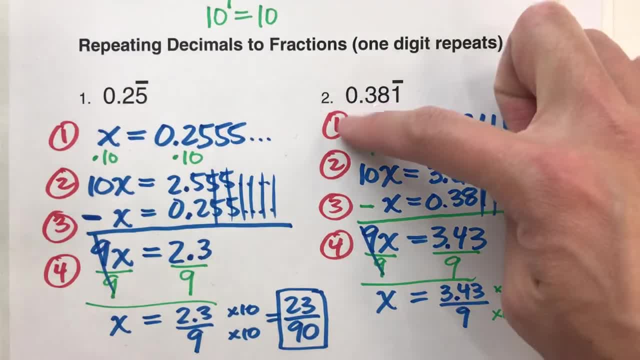 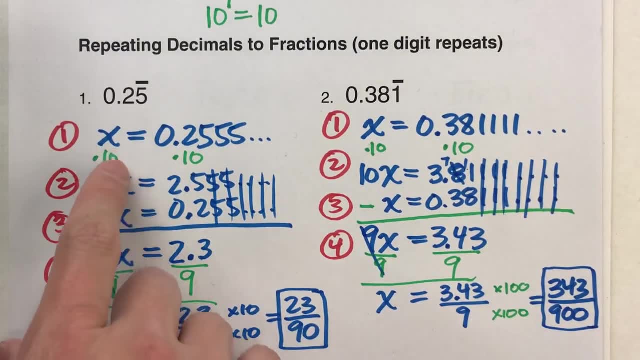 that is how to change a repeating decimal into fractions using four steps. all right, really, make sure you take the time to go through the steps. make sure when you subtract your equations, you line up those digits so that way, when you subtract them, you're subtracting the right numbers from each other. 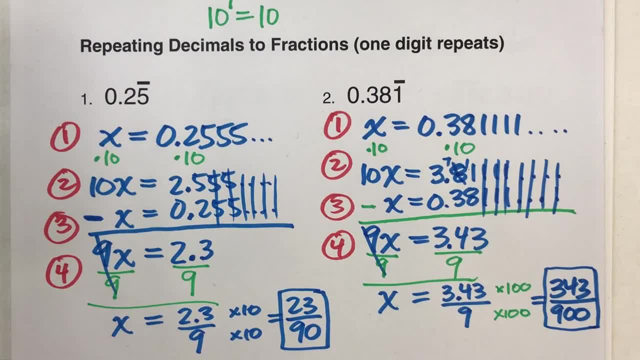 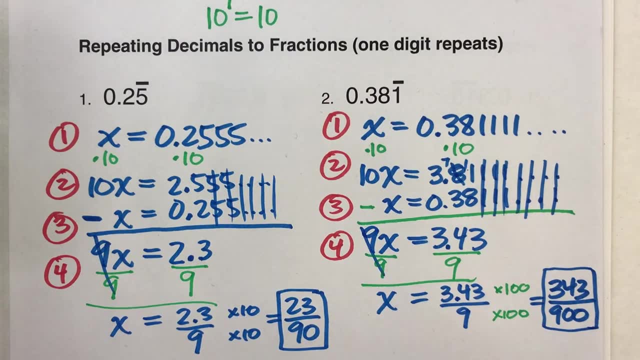 all right, work carefully, and thanks for watching this video. if you liked it, please hit that like button. also subscribe, because it really helps us out. but with that being said, good luck on your math, then i will see you next time. 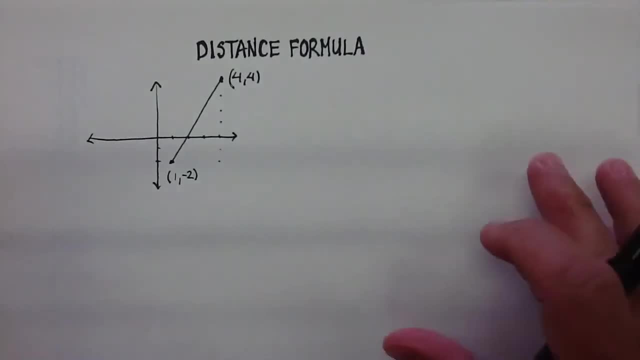 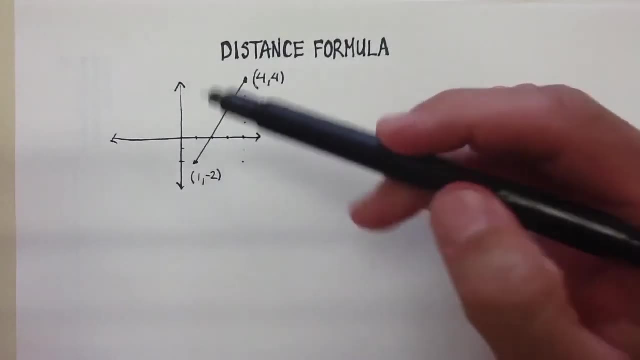 Okay, in this video I'm going to talk about something called the distance formula, And you use the distance formula when you have like a grid of some kind- x, y axis and you want to find the distance between two points that are not like on a straight line. okay, 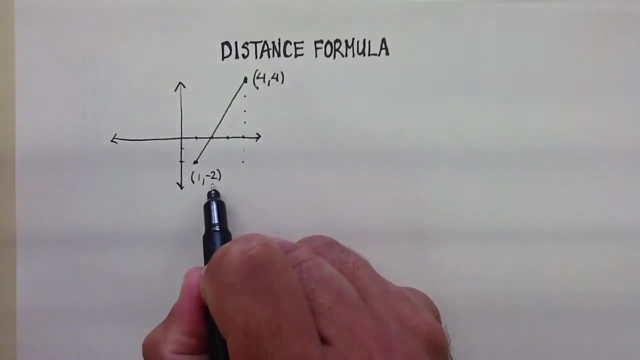 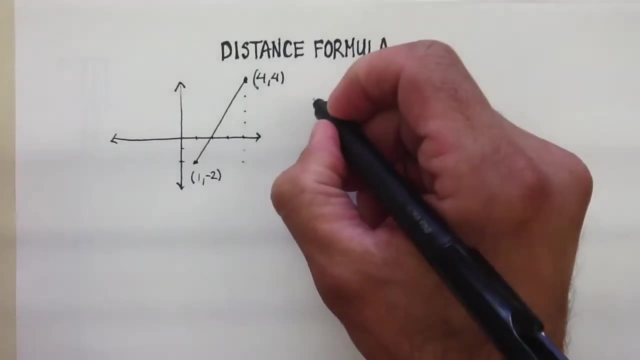 So, for example, what's the distance between this point here, which is 1, negative 2, and this point here, which is 4, 4?? And the distance formula is this. It is the square root. let me just write all this out.